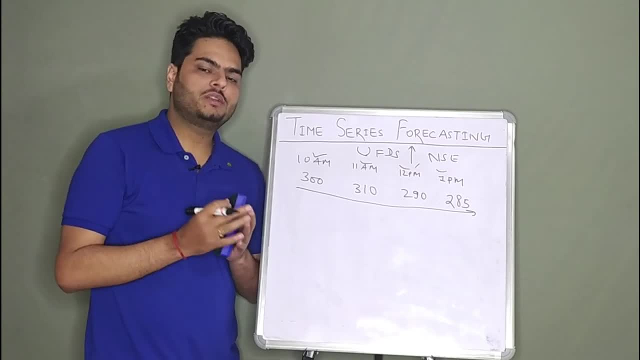 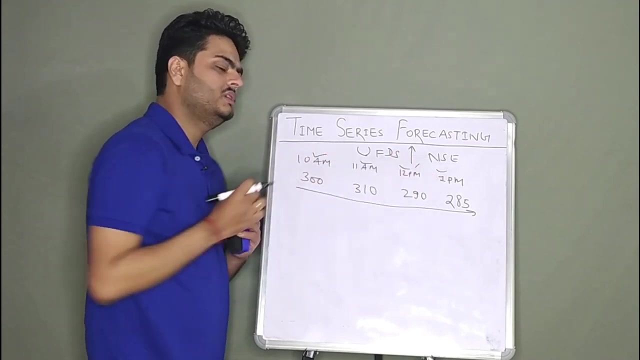 what can be the other example? the other example can be: if you are jogging or exercising, how many steps did you jog? how many steps did you jog before that day? wise capturing of that right. so all these kind of data where you capture the man, the magnitude, at different time intervals. 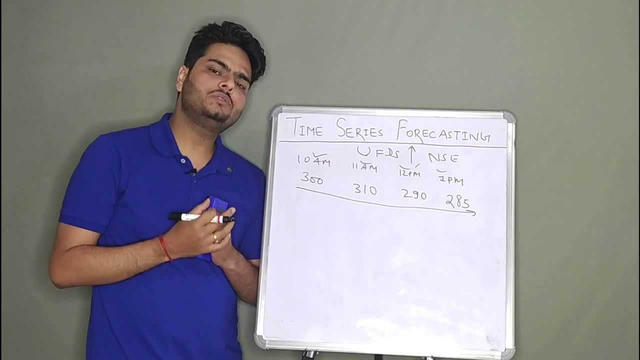 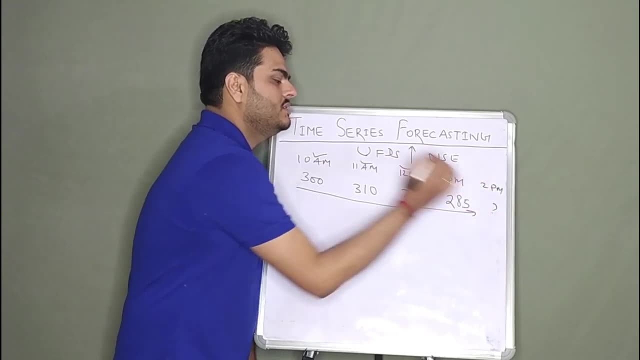 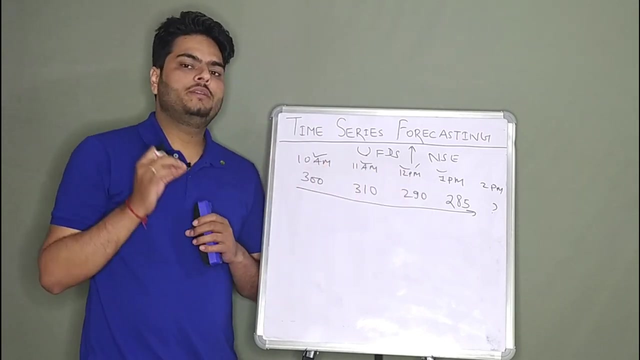 is known as time series data. what is time series forecasting? time series forecasting is: i give you this data and i tell you what will be the price of unfold data science at 2 pm. i tell you you are a data scientist, analyze this and tell me what will be the stock price at 2 pm. 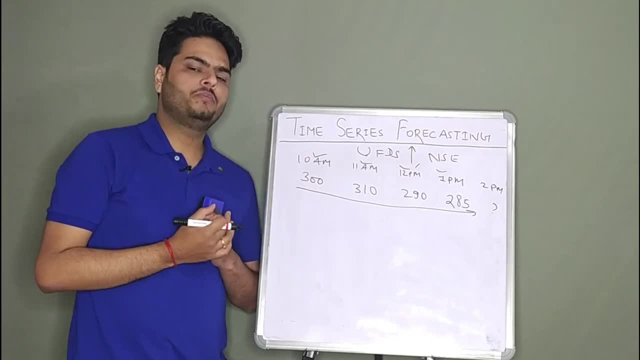 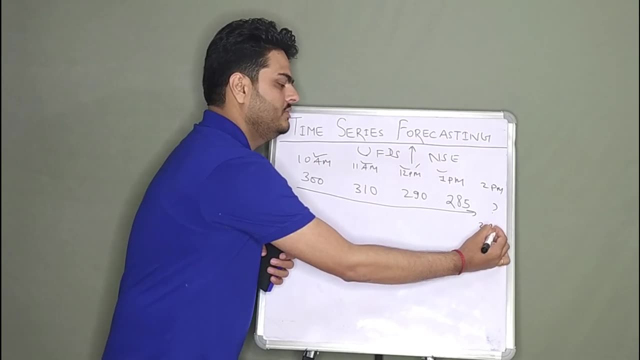 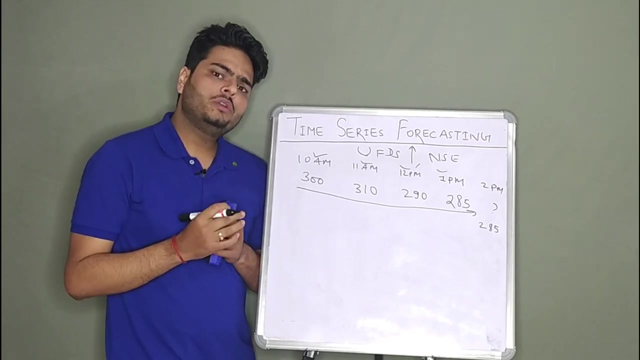 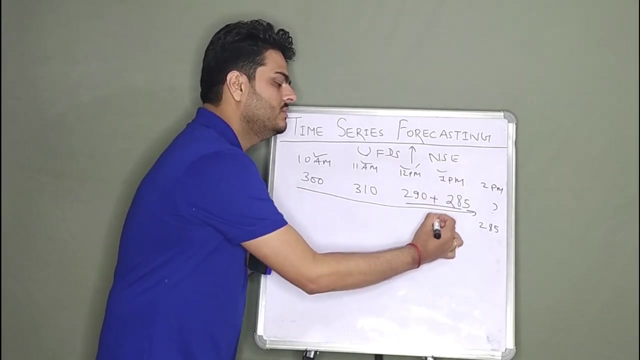 okay. so what can be the simplistic approach that you will take? you will say: you know what i feel. the price will not not change from one, so you can say directly: 285. very simple approach, okay. somebody can say: you know what i feel. why don't you take the average of two observations before? okay. so why don't you do average and just? 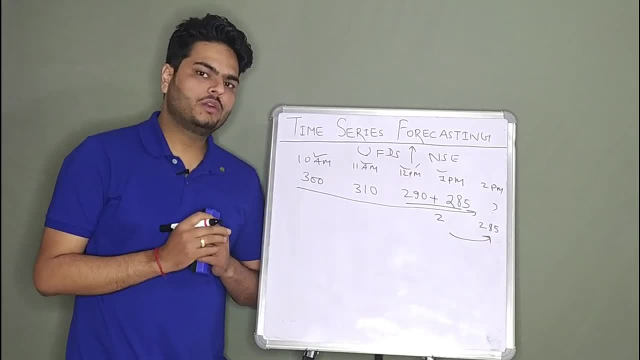 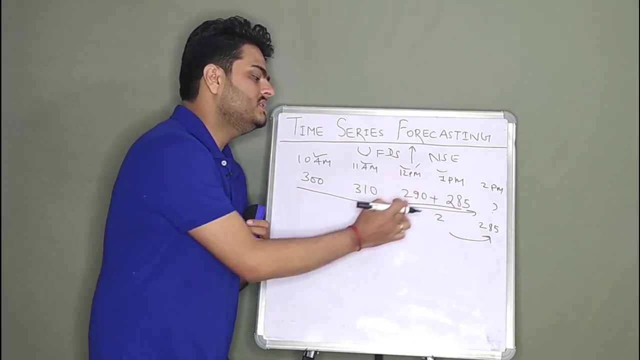 plug this number as a forecasted number. okay, somebody can say, hey, you are taking average means you are giving same weightage to both of these, but 285 is the more recent observations. hence, why don't you give more weightage to 285 and less weightage to 290? okay, the approach to that. 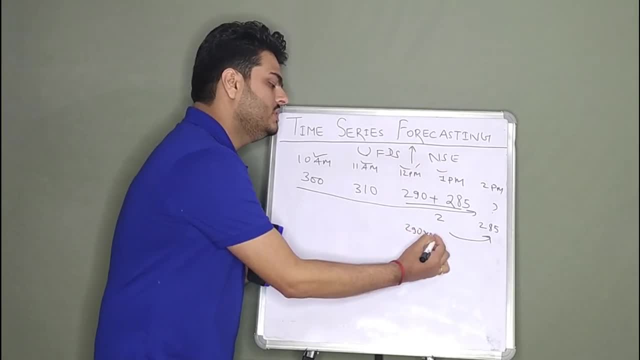 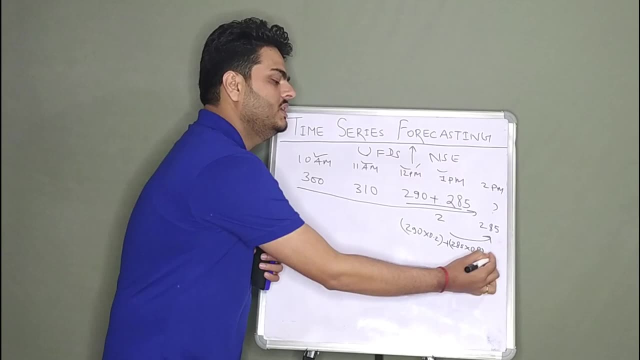 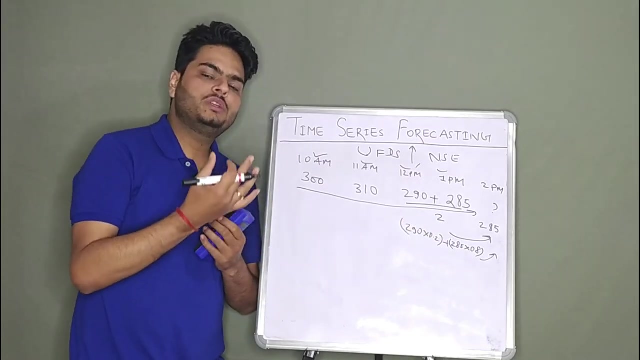 will be, let us say, 290 into 0.2, plus 285 into 0.8. this is the forecasted value. so what i am doing here, i am just dividing 100 percent between 20 and 80 percent. 80 weightage to the recent observation. 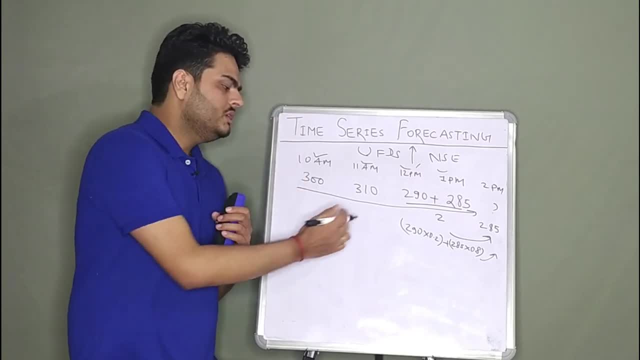 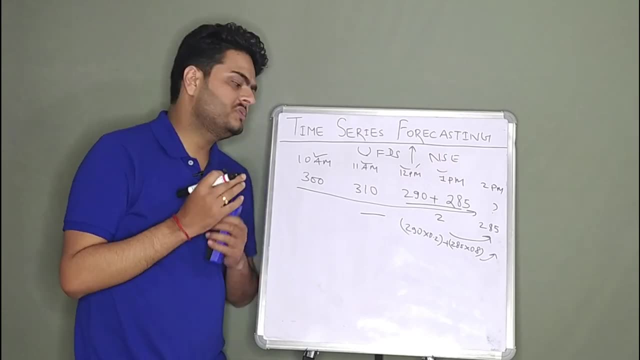 20 weightage to the before that observation. we can include this also and distribute the weight accordingly. these are some of the approaches which you take for time series forecasting. just some of the approaches i'm talking about. i'll go in more detail as well. okay, one important thing to 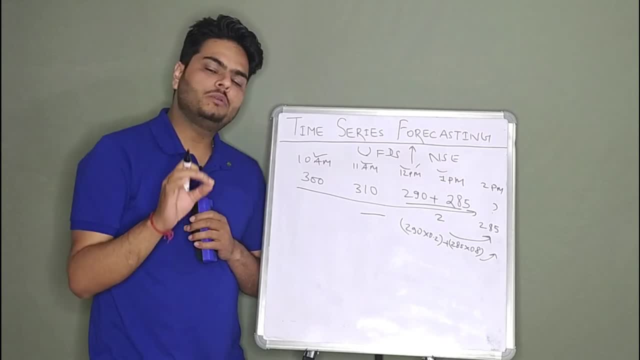 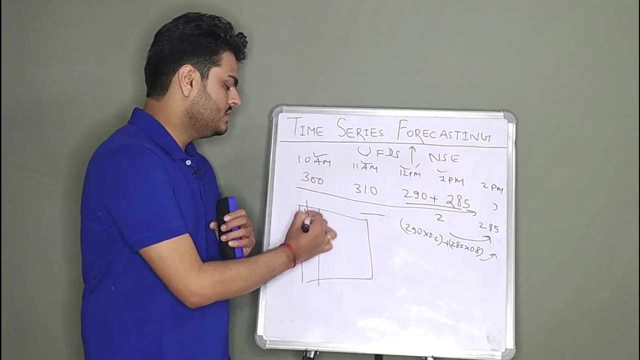 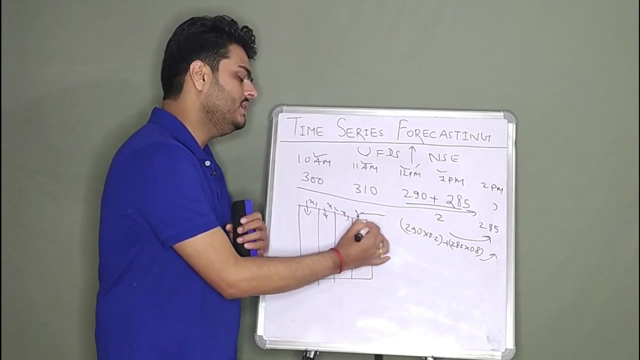 understand is how time series problems are different from traditional machine learning problem. so in traditional machine learning problem you will have a data like this: right, you will have x, x1, you will have x2 and then you will have a x3 and a target variable right. 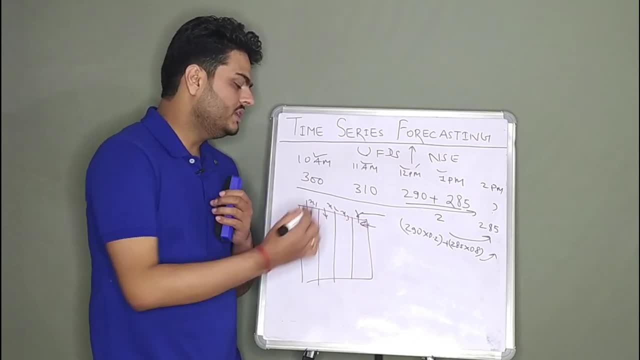 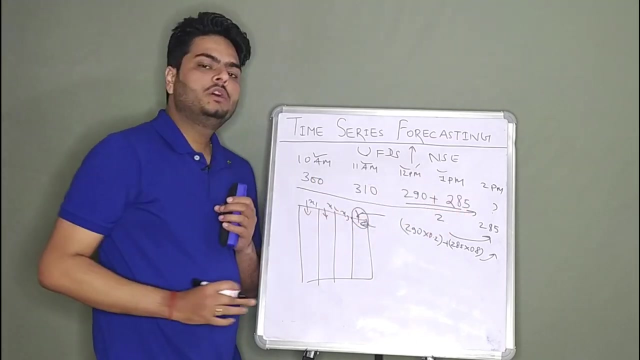 so how do you train your model? you train on your model, y model, such that y depends on x1, x2 and x3.. x1 and x2 and x3 are known as independent variables and y is known as dependent variable. Correct, In time series analysis you do not have any such. 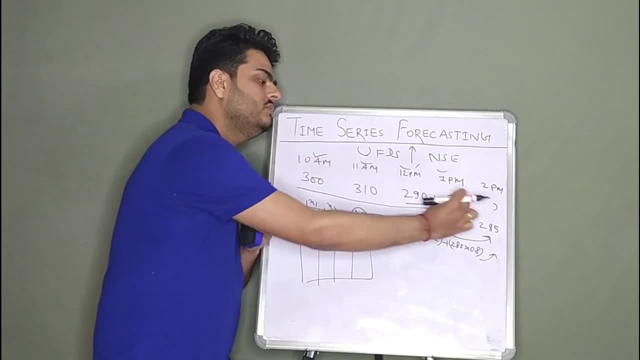 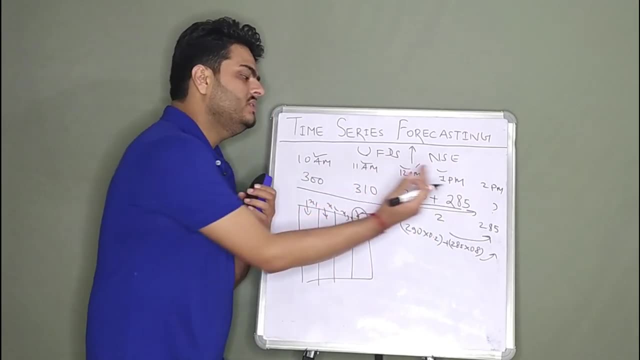 independent and dependent variables. What you have is just only one variable. So what we do, if you see, if you noted the examples, what I described, I just took the previous observations as deciding factor for the next value. So if I have to decide the next value, 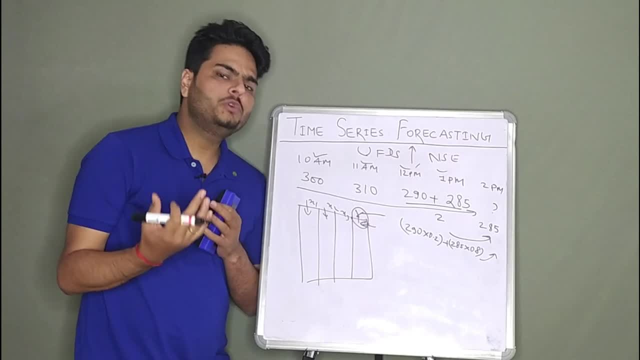 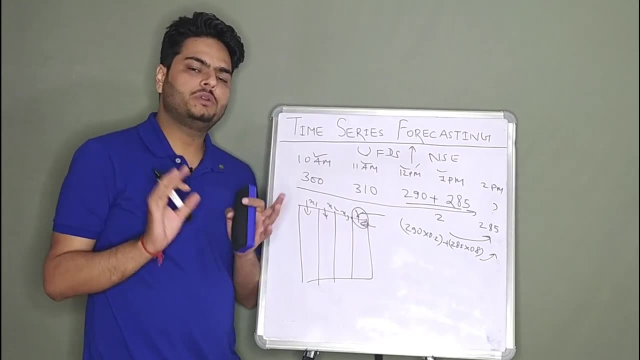 I just took the previous observations as the input for that, which means my independent features are nothing but the series itself. Okay, That is the basic difference between normal machine learning and time series. Here you have different, different variables. Here only one variable at different. 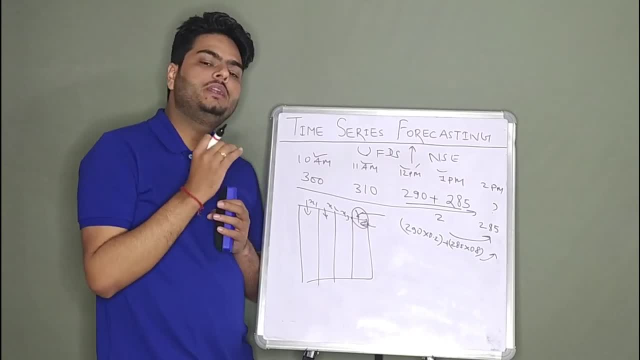 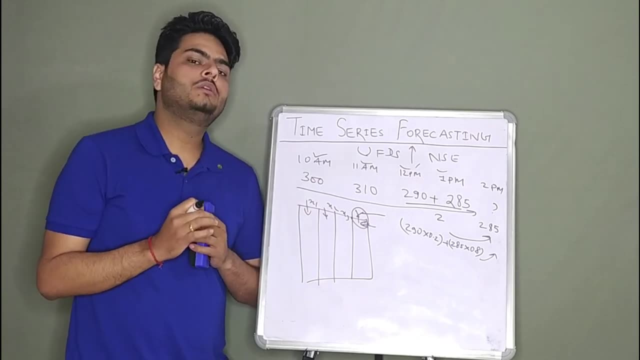 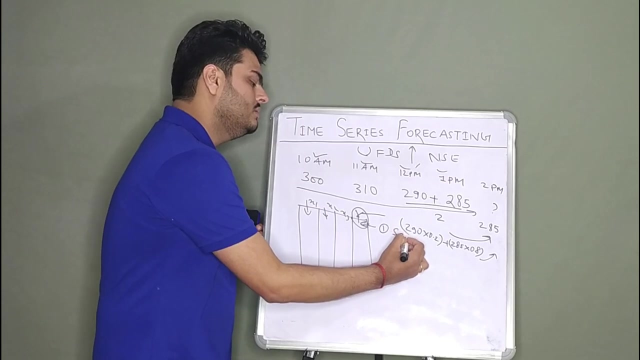 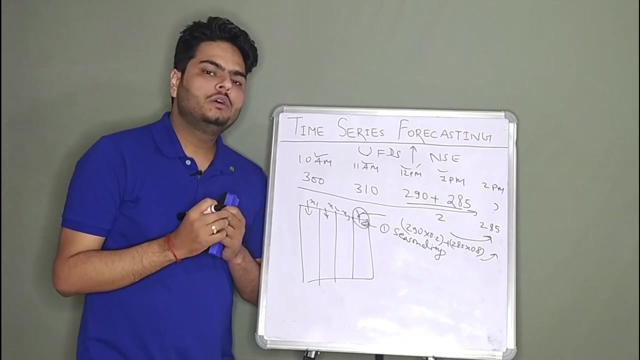 time intervals that act as your independent feature. Okay, Moving to next thing, what makes time series model difficult or a tough thing to work with? Okay, So the very first thing you should understand is something known as seasonality. Okay, So what is this seasonality? If you take example of any tours and travels company in USA, 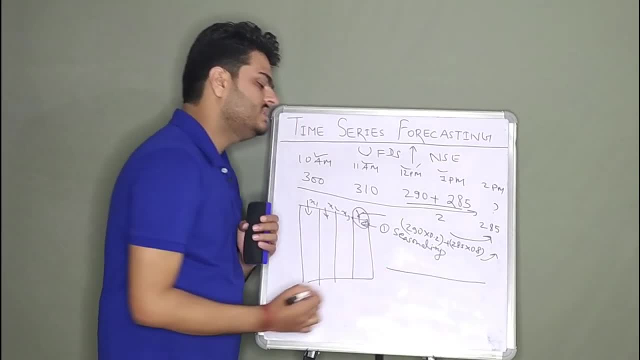 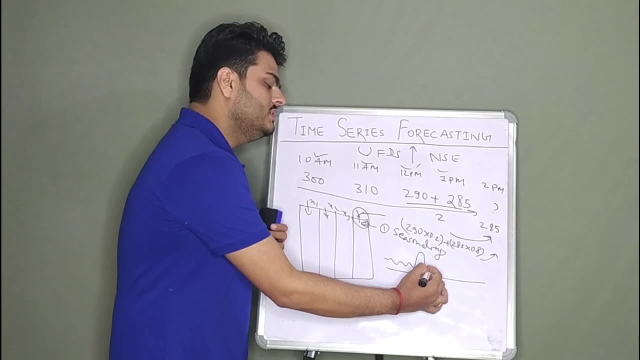 what you will see is, if this is the their sales data for last three years, right, Then you will see that it goes like this, And every year in the December it peaks like this: Okay, The reason for this peak is nothing but. 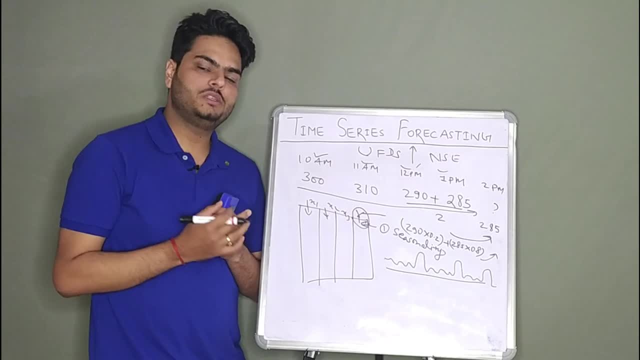 it is a holiday season, right, It is a Christmas season. Hence, every year in December, you will see a peak like this. This is called seasonality of time series. So when you are working with time series data, you have to capture this seasonality, Otherwise you will not be able. 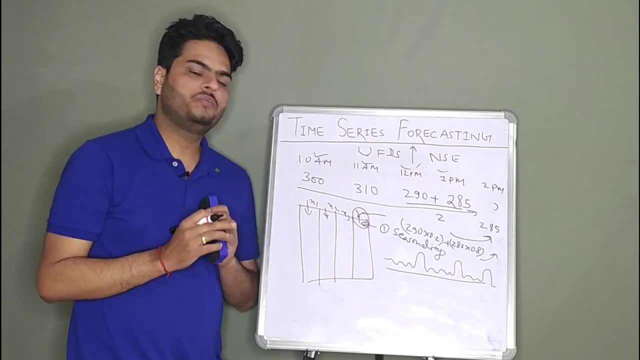 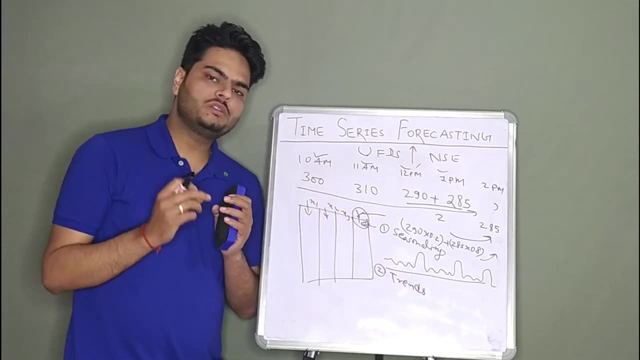 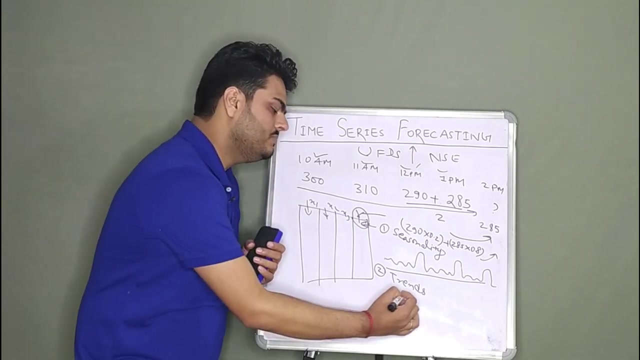 to give proper forecast right. This is seasonality. The second thing you have to understand is known as trends. So what is trends? Some companies, over the period of time, might be in an upward direction, their revenues, For example. if I in this chart. 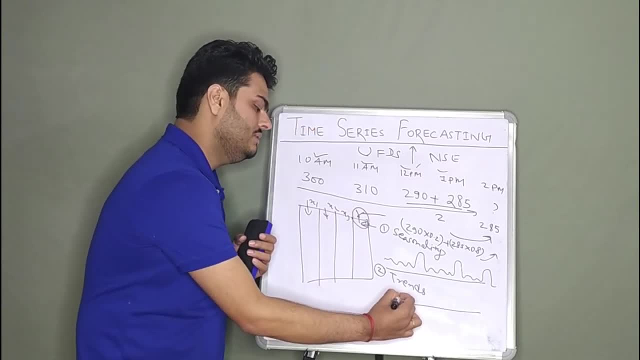 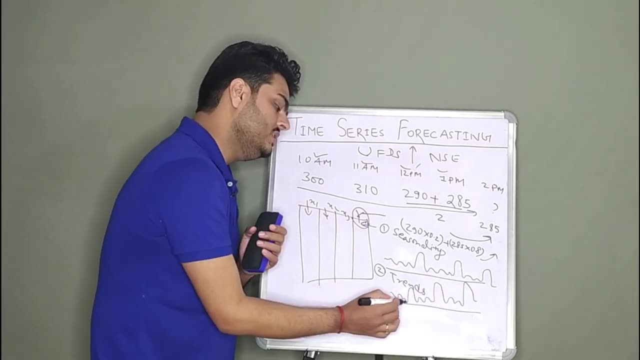 also, I can draw this chart like this as well. right, There is a seasonality, but at the same time, the chart is also going up. So, if you see, the chart is going up like this, which means that 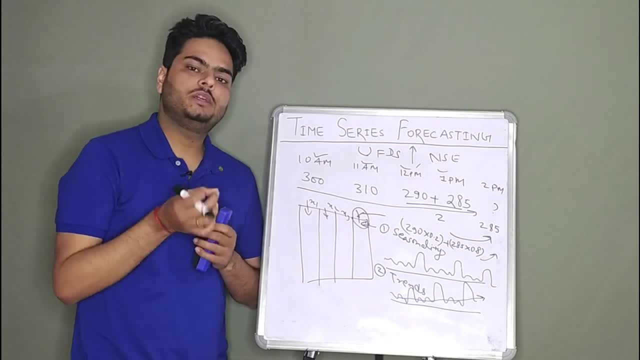 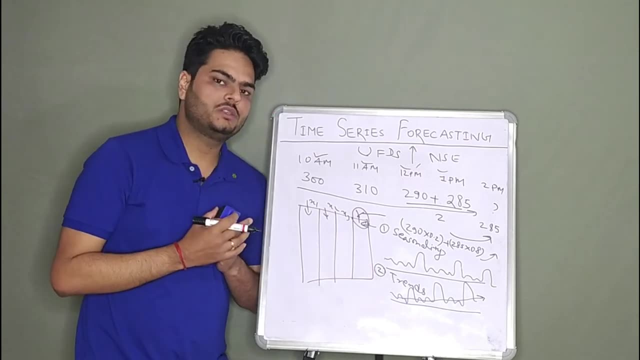 the trend is also going up according to the seasonality. The third things is: what is there in terms of segúnality? In addition to seasonality, there is an upward trend also. This is known as the trend component of the time series, of time series: right Seasonality. 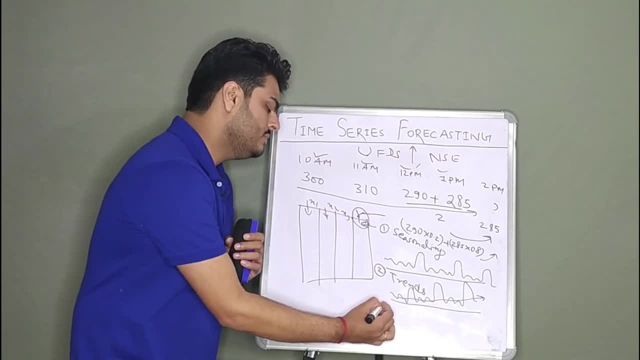 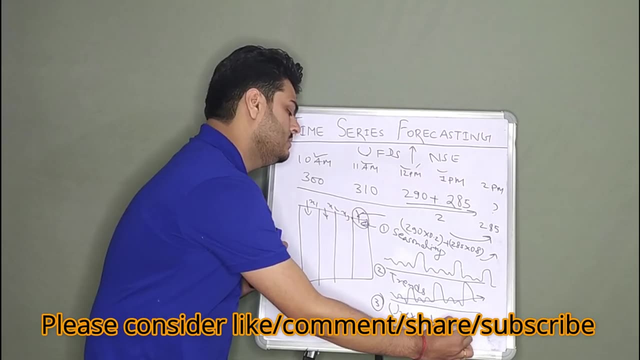 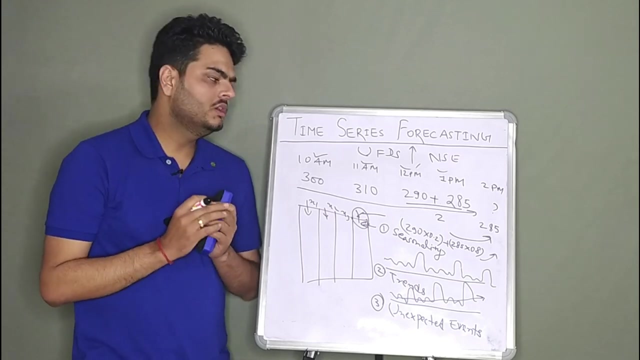 and trend, two basic components. Third, Things-unexpected events. Unexpected events: What is the unexpected events? Something like what we are going through now, right, Something like what you are going right. so if you see the sensex or nifty chart or any stock market chart, you will see a huge dip in. 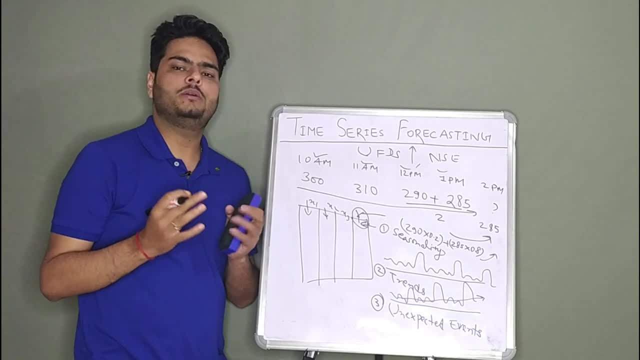 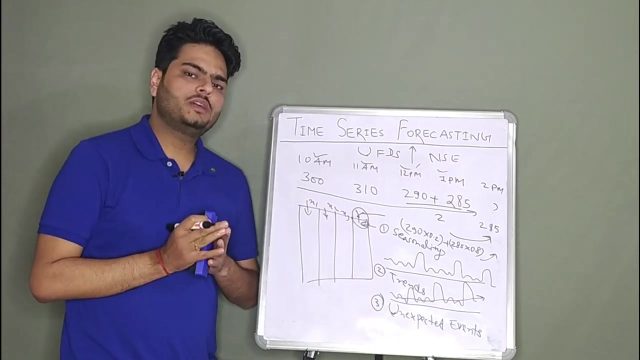 the month of march and april 2020. the reason for that is the current pandemic right. so these kind of situations, whatever time series forecasting you do, the future events might not get captured. if there is a future uncertain event or unexpected event, right, but in the past, if there are some. 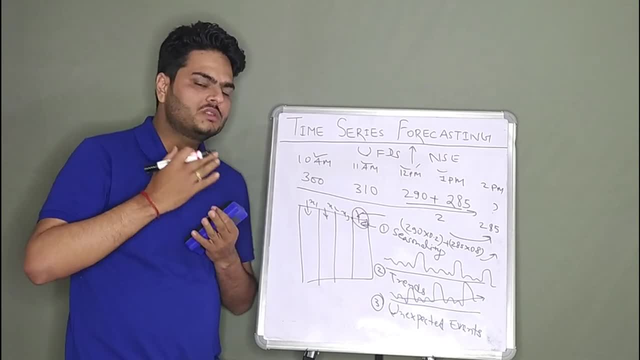 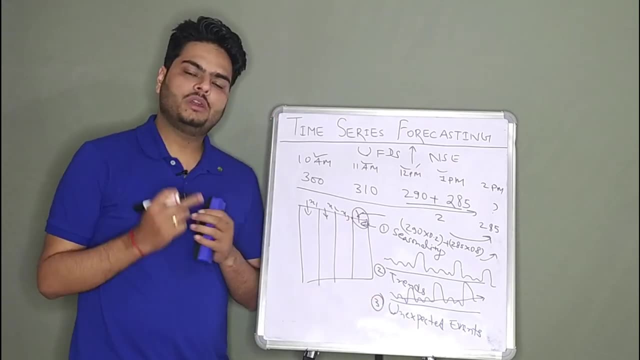 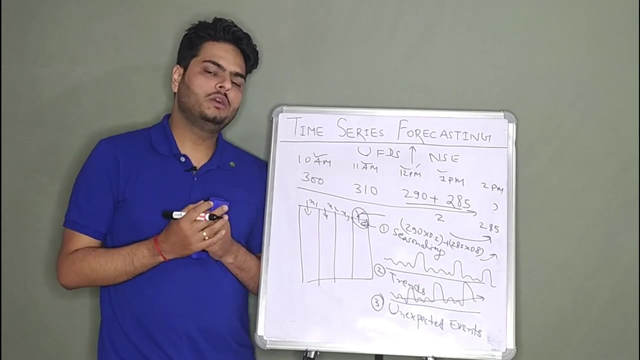 unexpected event which has occurred- for, like you know, sometimes there is a regularity in that- then at least we can capture, but unexpected event capturing this becomes very, very difficult. okay, so these are some of the things that make your time series model or forecasting little tricky or little difficult. there are packages available, there are techniques using which. 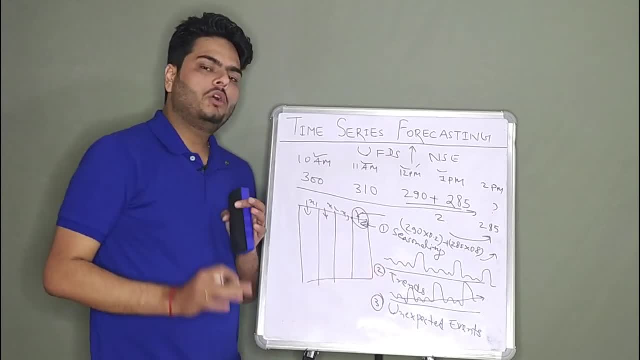 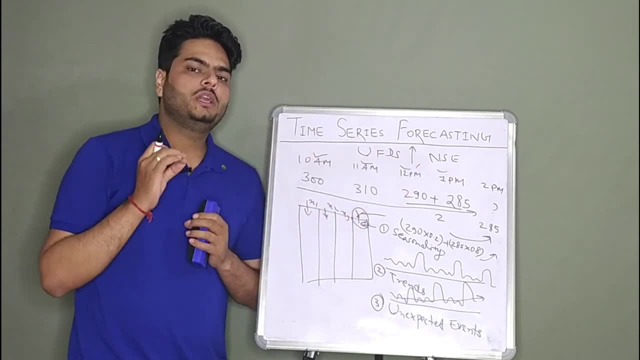 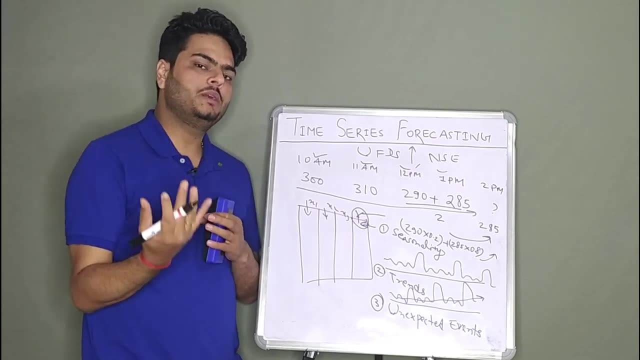 is showing and you can forecast the future value. okay, in my next video i will continue on different different applications of time series, different different data models that we use to work with time series, and i will also show you in practical, in python, how to work with those packages and 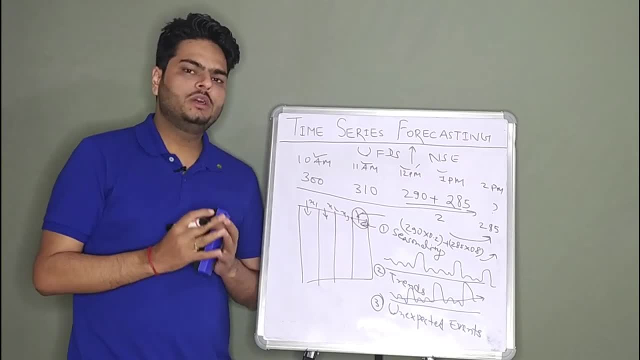 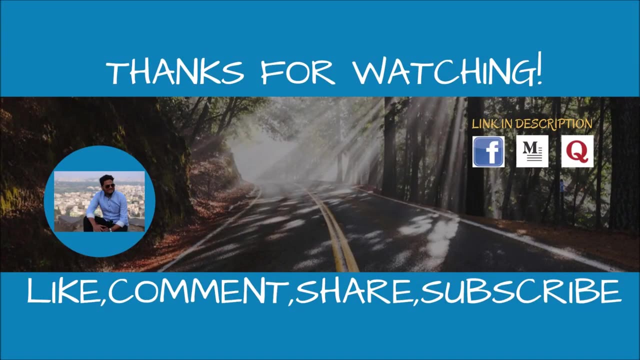 those functions. if you have any doubts here, write me in comment. i'll see you all in the upcoming video. till then, stay safe and take care you.